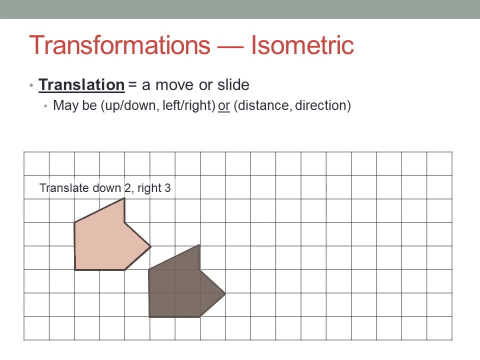 The image will be congruent to the original object, But every point of the image will be two down and three right of where it was before. If, instead, I ask you to translate the shape a distance of seven squares in the direction east-northeast, then it's a little bit trickier. 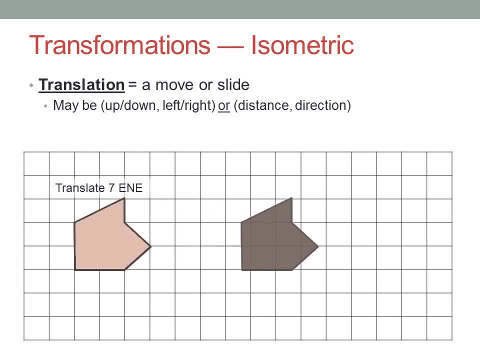 First find where the distance of seven is. That'll put it somewhere on a circle of radius seven. Now all we have to do is get the direction correct. It's halfway between east and north-east at twenty-two and a half degrees. 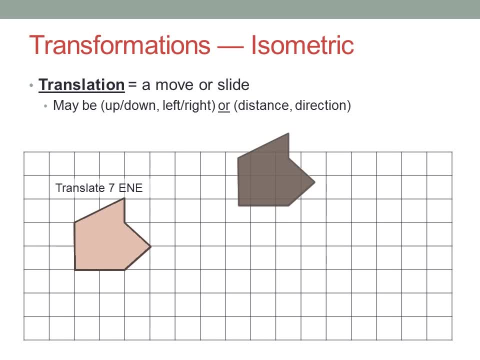 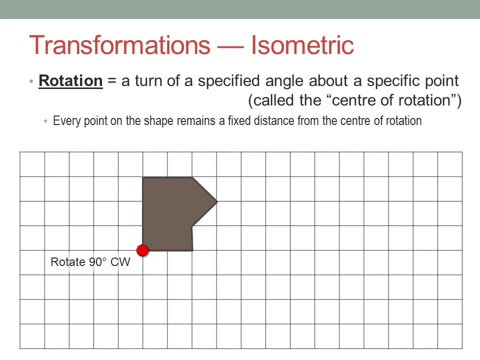 The image is congruent to the original object, but every point of the image is now seven squares distance away east-northeast of where it started. A rotation is a turn of a specified angle about a specific point called the centre of rotation. The centre of rotation must always be specified. 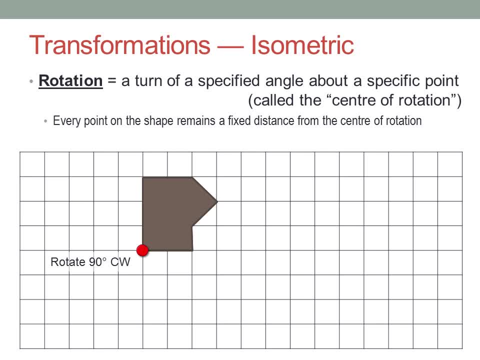 Every point on the shape will remain at the same fixed distance from the centre of rotation. For example, let's rotate this shape around the marked centre of rotation at the bottom left of the shape. We'll rotate it ninety degrees clockwise. Sorry, even if you prefer digital watches, you still need to know which way clockwise. 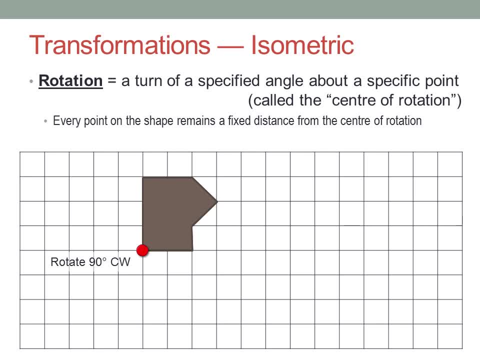 or anti-clockwise is. The easiest way to do this is actually to cut the shape out of another piece of paper. Then you can literally hold the bottom left corner still and rotate the cut-out shape around it. We want a quarter turn clockwise. 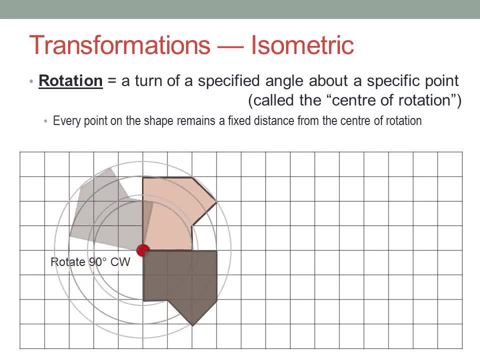 Did you notice, as we rotated it, that each part of the shape turned clockwise? Did you notice a shape moved in a circle around the centre of rotation? Every point in the image is the same distance from the centre as it was in the object. 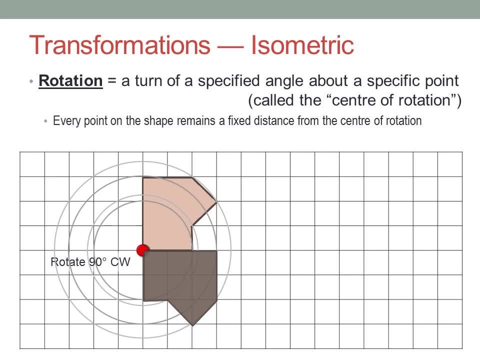 But the centre of rotation doesn't have to be part of the object. Here's an example where the centre of rotation is off to the right. We have to rotate it anti-clockwise ninety degrees. This is a little trickier, but again, let's make this one a bit more complex. 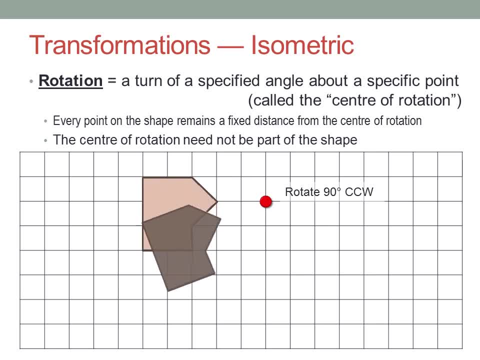 Let's go back to the drawing board. Let's get our cut out shape and rotate it around. Can you see the circles? each point on the shape is following. Where are they centred? It may help you, if you're cutting the shape out, to include the centre of rotation in. 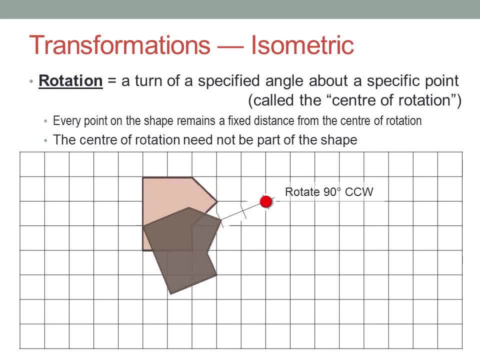 the piece you cut. Then you can hold it still there as you rotate. And of course the angle of rotation need not be 90 degrees. This one says to rotate 45 degrees clockwise. Getting the distances and positions right can be a bit harder. 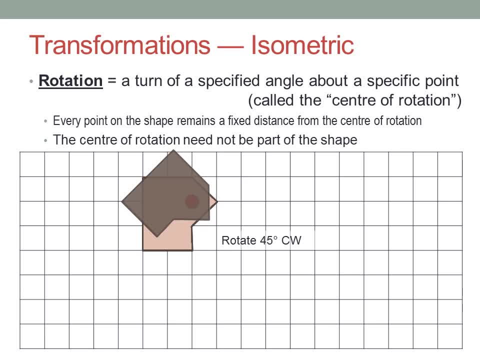 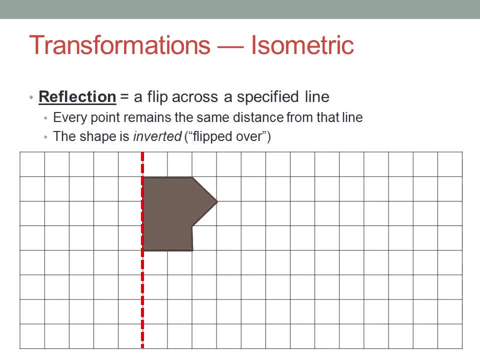 I really recommend you cut the shape out and literally pull it around. It really will help you. A reflection is a flip across a specified line. Every point in the shape will remain the same direction. There is no distance from that line. but on the other side. 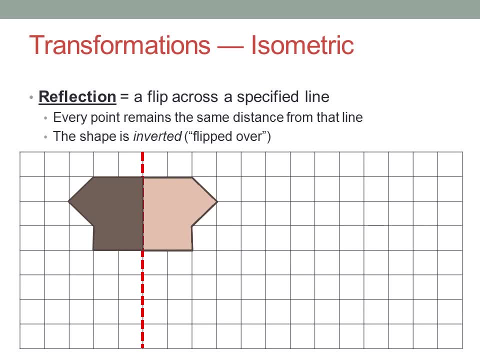 When the line is vertical or horizontal. it's usually fairly easy to do. The image is inverted, but we still say that it's congruent to the object. It's flipped over, but the angles and lengths are all still the same and are still in the 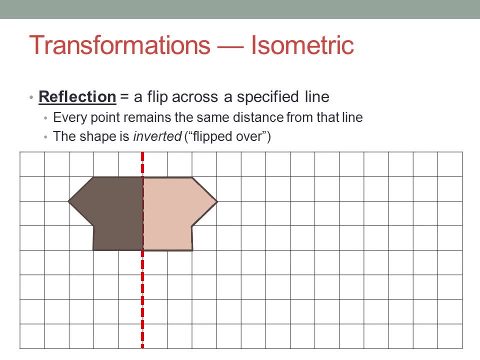 same relationships with each other. A flipped over shape, an inverted shape, is still said to be congruent, But if the reflection line is at a different angle, it can be a bit trickier. What you have to do is use the definition of the reflection to work out where the image 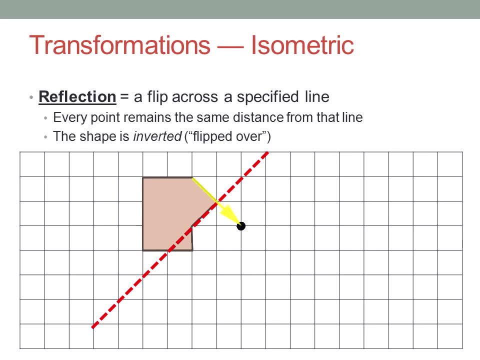 is, Each point is the same distance from the line, but on the other side Any part of the shape on the line doesn't move, but every other point gets moved directly across the line to the same distance it was on its original side. 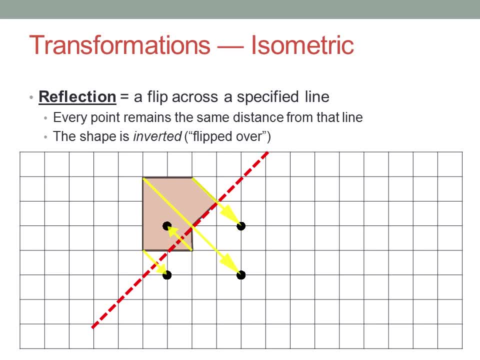 Even points on the other side get moved across the line to the same distance they were See, And the resultant image will be congruent to the object, but inverted Again. if you prefer, you can cut the shape out and literally flip it over. 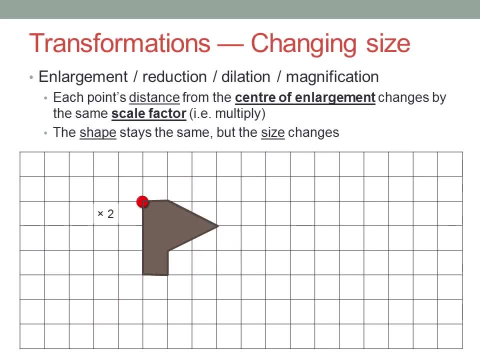 Finally, transformations that change the size of the shape. This is variously called enlargement, reduction, dilation or magnification. Generally, enlargement is for making the shape bigger with a scale factor greater than 1, and reduction is for making it smaller with a scale factor less than 1.. 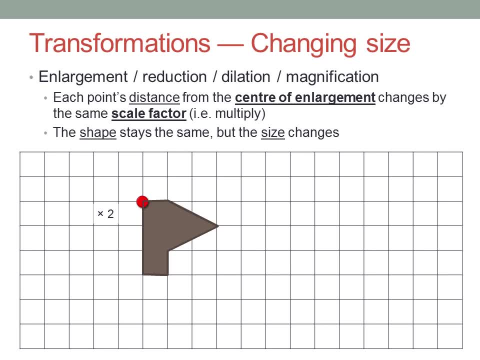 However, the terms are more or less interchangeable. Each point in the shape has its distance from the centre of enlargement changed by the same factor called the scale factor. The word factor should remind you to multiply the length by the scale, The angles in the shape will stay the same, but the size will change. 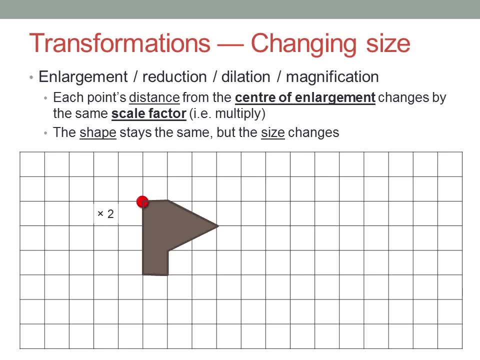 Every side's length will be bigger or smaller by the same scale factor. This is what you can do with a cutout, because you can't really stretch the paper, So instead you'll have to work out the points separately and then join them up. 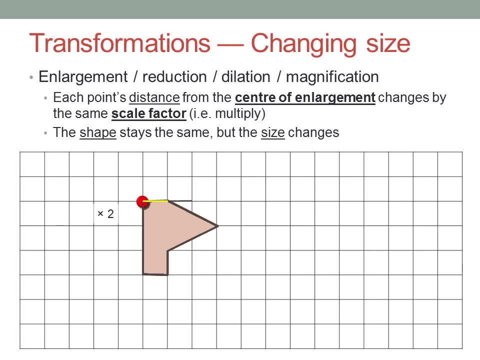 Take each point and, in this case, double each distance away from the centre of enlargement. See how it works, The trickier ones just do carefully. Double the vertical distance and double the horizontal distance And there's the image. It's twice the size, but the angles and relationships haven't changed. 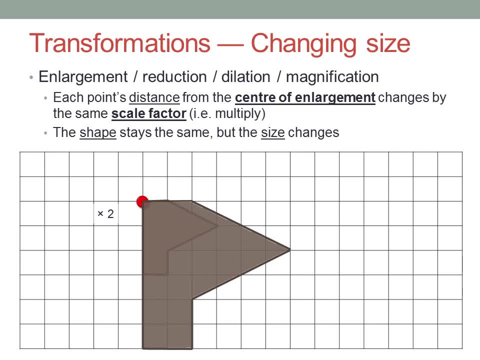 We say the image is similar to the object: The same angles but not the same lengths. It's similar but not congruent. Let's try a reduction where the scale factor is smaller than 1. Here every point's distance from the centre has to be reduced to one third of what it. 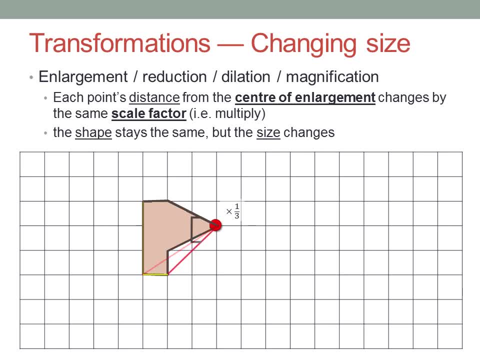 is Lightly draw in the lines from the centre to each point and measure one third of the distance, Then connect them up And there's the image, Exactly one third the size of the original. And of course the centre of enlargement doesn't have to be part of the shape, just like when